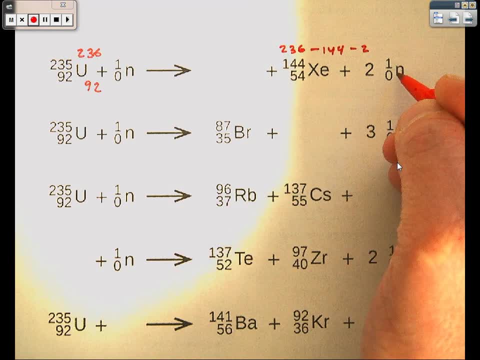 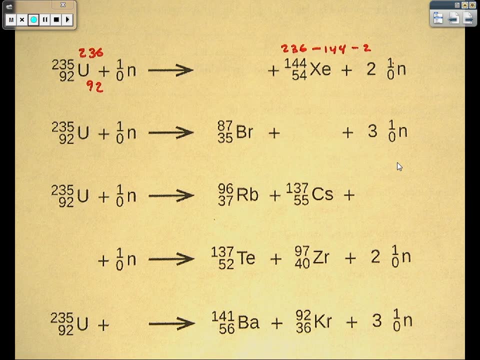 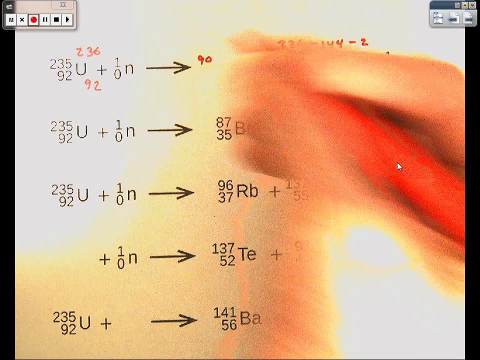 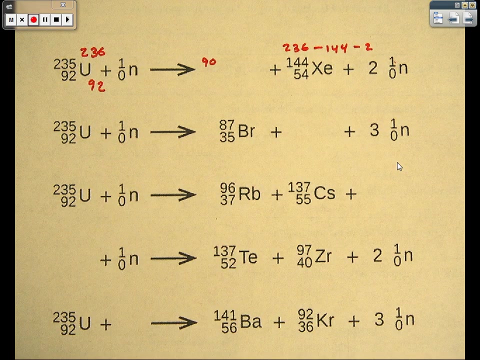 minus 2 from the neutrons. 2 times 1 gives us that 244.. We're going to subtract there, So 236 minus 144 minus 2 is 90. The missing mass, the mass of our unknown substance, has to be 90 in order to keep the mass the same on both sides. We'll do the 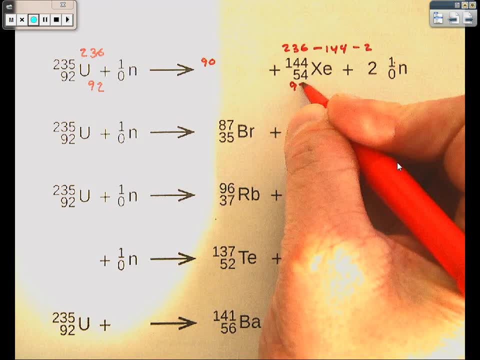 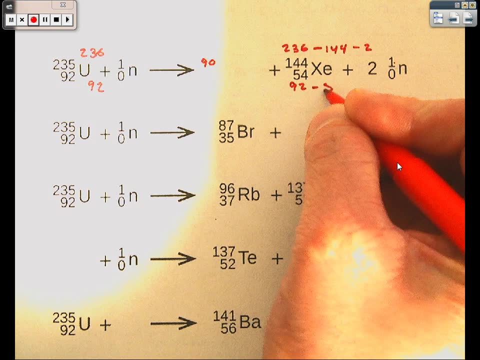 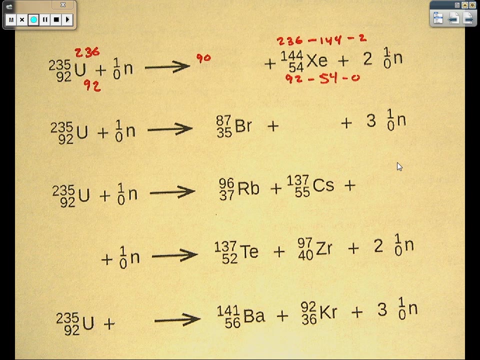 same thing with the atomic number. We'll start with 92, the mass from the starting side. Subtract out the 54 from the neutrons. We'll subtract out the 54 from the neutrons. We'll subtract out the 54 from the xenon And 0, 2 times 0 for the neutrons. So 92 minus 54 minus 0 is 38. That's. 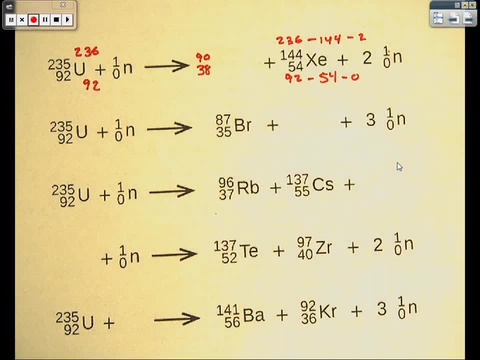 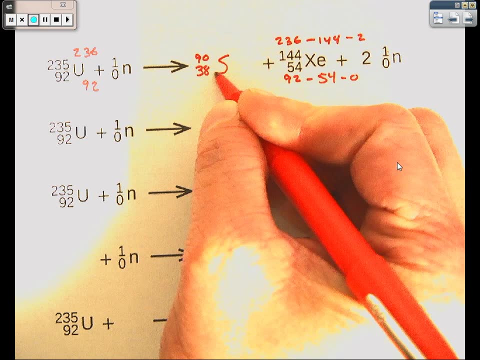 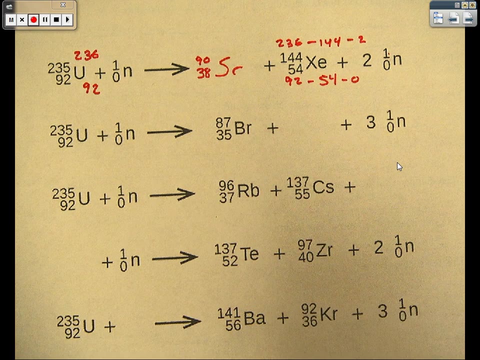 the atomic number of our missing substance. As always, we look up the symbol based on the atomic number. We look up the symbol based on the 38.. Number 38 on the periodic table is strontium Sr. We're going to do the similar kind of process with every kind of problem. We're going to look at what. 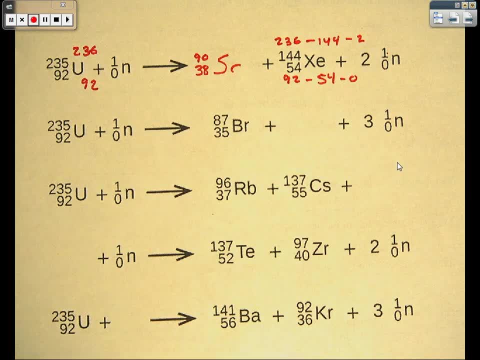 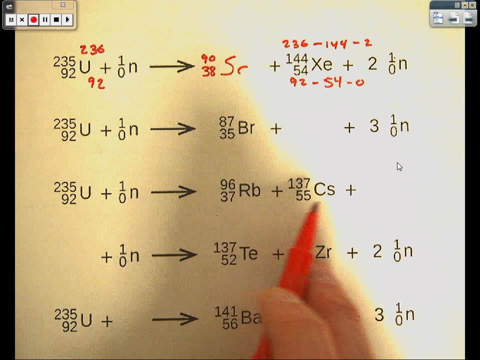 the total mass is on the complete side. Subtract out what we have on the incomplete side to find the missing part. This third one is set up a little differently, because we know the two product atoms that are going to be produced by the fission of uranium. What we don't know is how. 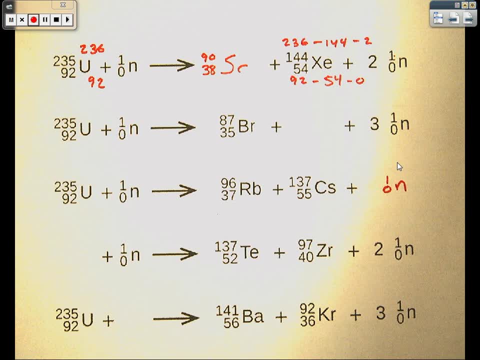 many neutrons. We know there's a 1,, 0, n that belongs here. We know there's neutrons being produced, We just don't know how many. We know there's a 1,, 0, n that belongs here. We know there's. 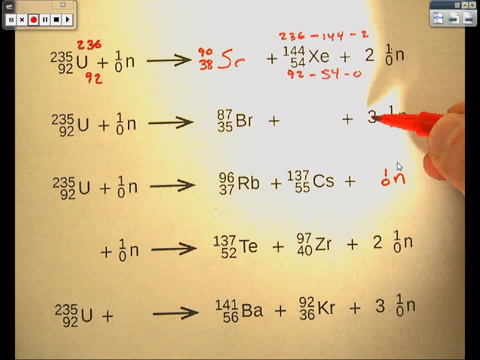 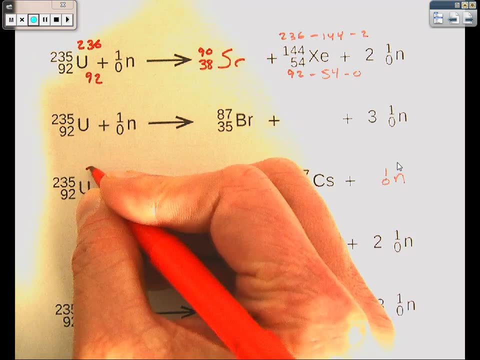 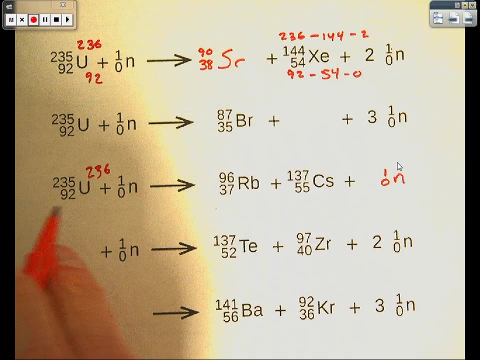 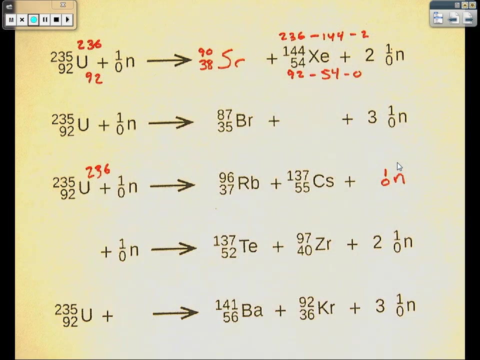 a, 1,, 0, n. that belongs here. We have to find this coefficient that goes out front, And we're going to do it the same way we did the first one. We're going to total up what we have over here on the starting side, That's 236 for our mass. We're not really concerned about atomic number this time. We have a total of 92 over here. We already have a total of 92 over on our product side. So all we're concerned with is really the mass. We have 236.. We need 236 on this side. 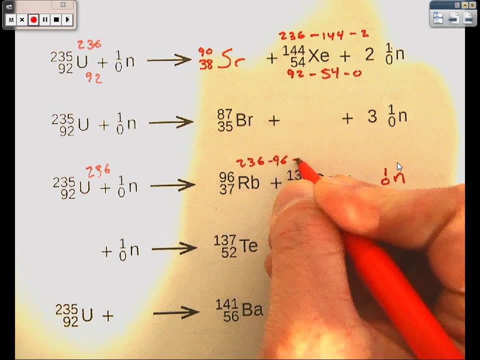 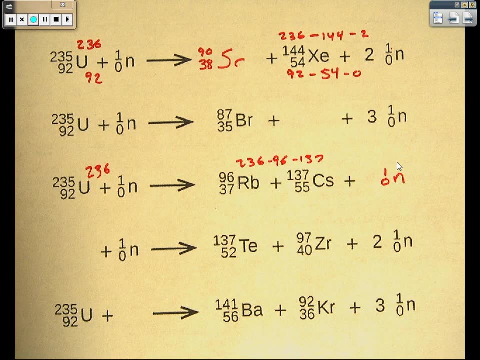 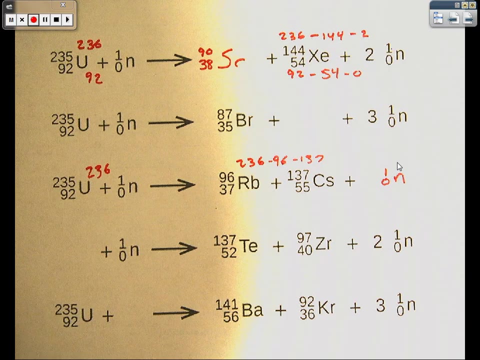 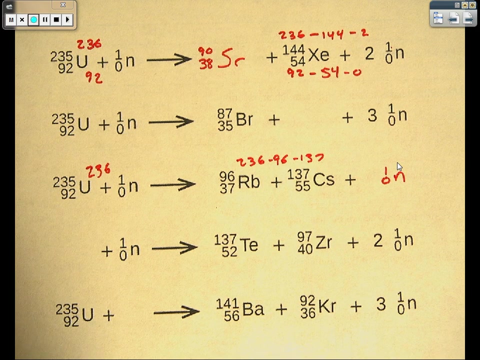 So we'll take the 236 minus 96 minus 137.. The 96 from the first element, the 137 from the second one. We subtract that out, We get 6.. 236 minus 96 minus 137.. I knew I punched that in wrong. Let's get 3.. 3 is the number of neutrons that have to be produced. 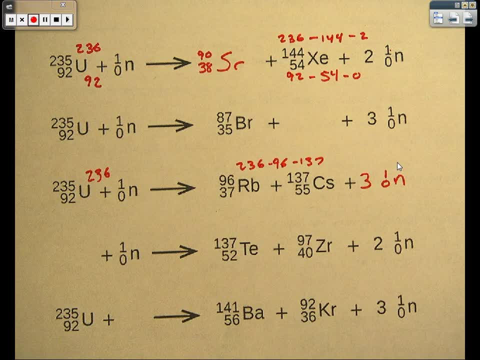 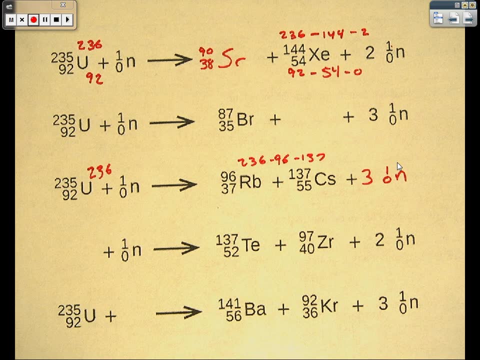 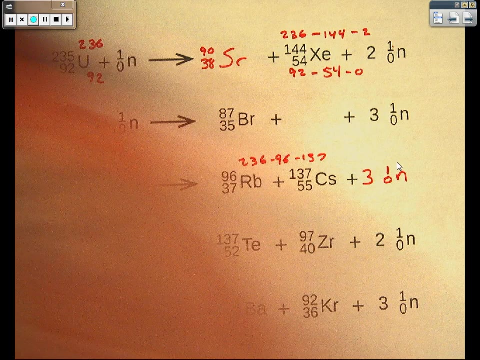 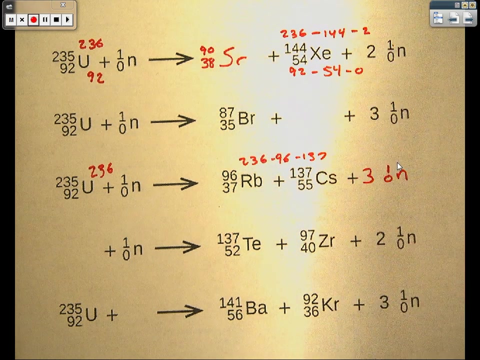 in this fission reaction, Even if we're working back over towards the starting side. same principle: We're going to add together everything we have on our complete side. This time we're going to add together everything we have over here on the right. So we have 137 plus 97 plus 2.. Again, 2 times 1.. This is 236.. 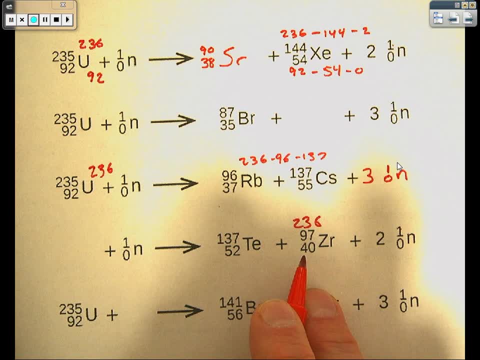 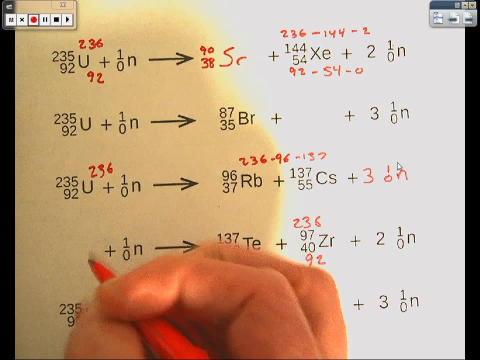 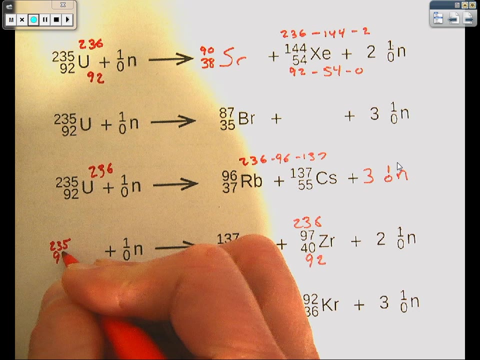 52 plus 40 plus 0 is 92. And subtract out as we go the other way, So 236 minus 1.. 235.. 92 minus 0.. 92.. Look up 92 on the periodic table. That's your ring. 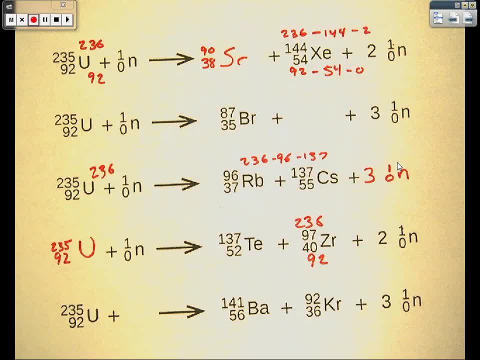 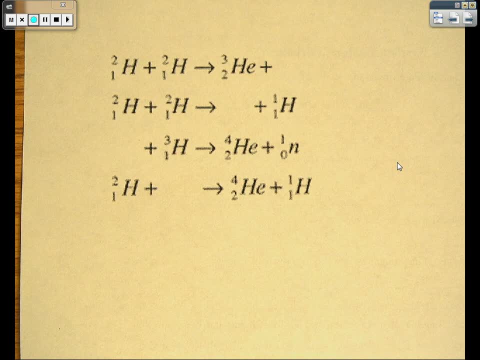 Those are the fission equations. The fission equations are going to be solved using the exact same principles. We know that the total of the mass on one side has to be the same as the mass on the other. The total of atomic number on one side has to be the same. 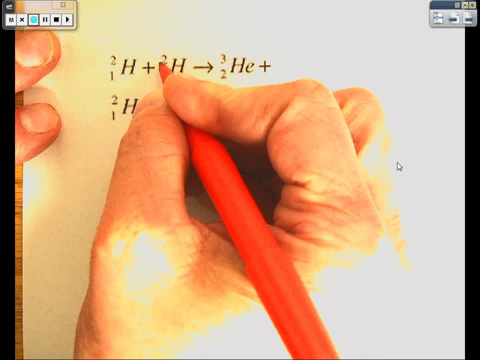 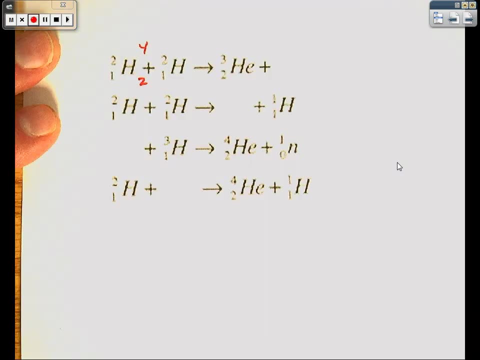 as the atomic number on the other. So again, add up your complete side. 2 plus 2 is 4.. 1 plus 1 is 2.. Subtract out what you have on the other side. So we're going to do 4 minus. 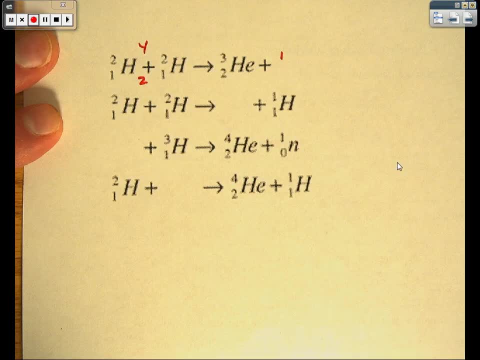 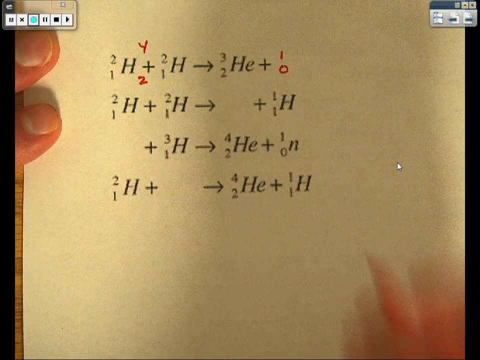 3. We have a mass of 1 left on that second part. 2 minus 2 is 0.. The only thing we have with a mass of 1 and an atomic number of 0 is the neutron. to put there, This is producing a neutron.